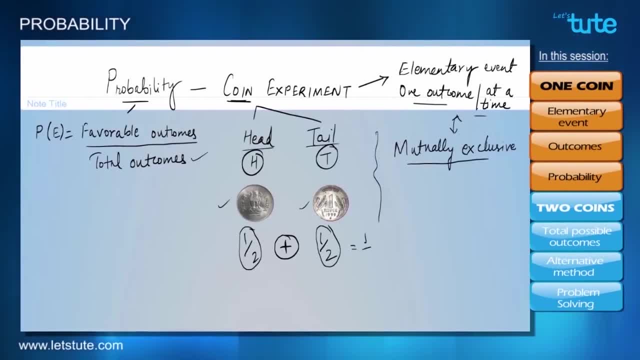 remember, when we say mutually exclusive, we add. So when we are adding probability of head with probability of tail, we get a total probability of 1. That means it actually satisfies the sum of probabilities rule as well. And moreover, we see: 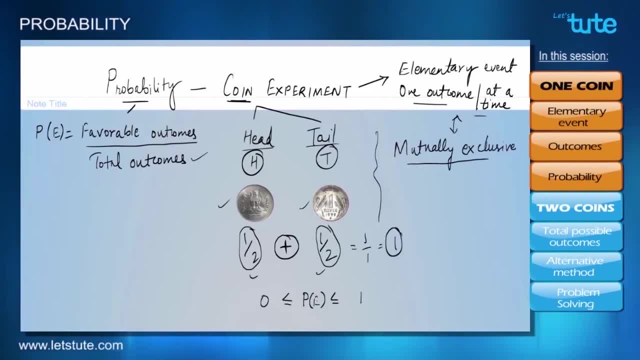 that 1 by 2 lies between the extreme probabilities of 0 and 1.. So the event of coin tossing actually satisfies all the probabilities rule. How about making it more interesting and talking about probabilities associated with two coins? Let's name our coins as A and B. 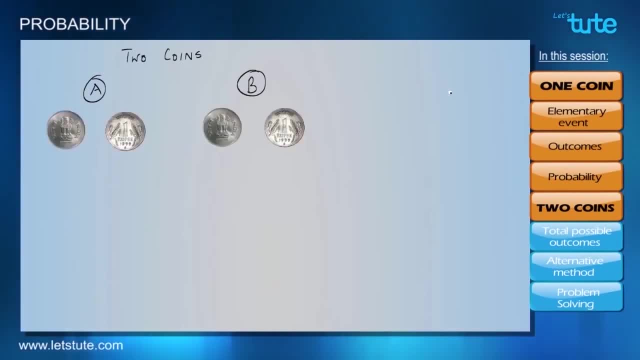 And each of them will have same outcomes, heads and tails. Now, in order to know the possible outcomes from the event of tossing two coins, what we'll do is we'll group outcome from coin A with the outcome from coin B, And this particular set will be the outcome of tossing two coins. So, 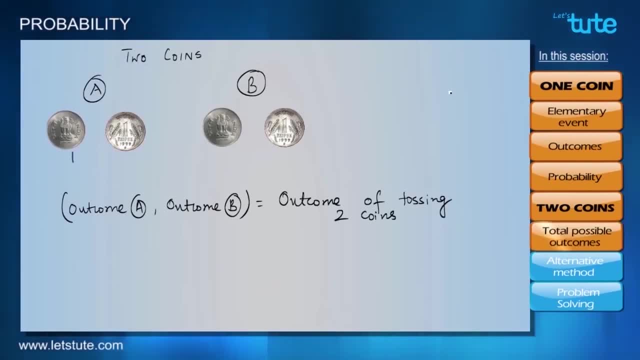 let's say, upon first time tossing we get heads on both the coins, that is, H and H. So we'll write H- T. Upon second time tossing we get heads from coin A and tails from coin B. Then we'll write H T. 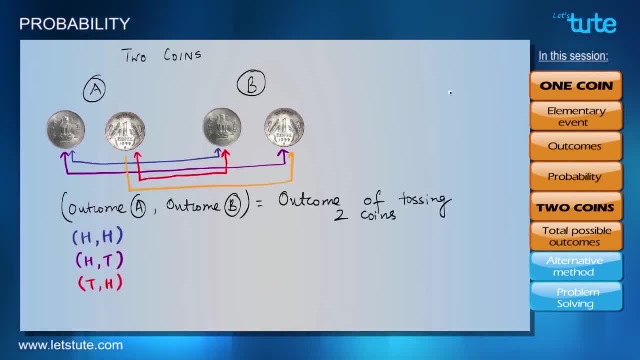 Similarly, we can write all the possible outcomes. So you can go ahead and try tossing two coins and see if there are any more possible outcomes that can appear, And you will see that there are only four outcomes that are possible. Now there is a faster way of actually calculating. 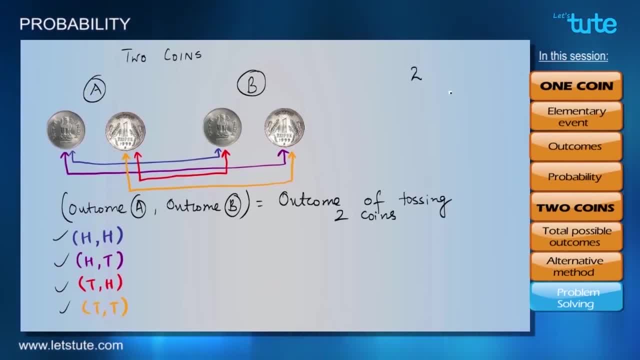 the total possible outcomes. We know that there are two outcomes of a coin tossing: heads and tails. So if you are tossing it once, then we write it as 2 raised to power, 1, which is equal to 2. so the power actually signifies the number of times events take place and the base actually. 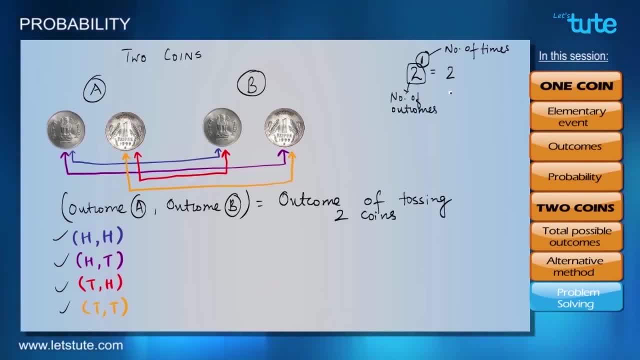 tells us the number of outcomes of an event. similarly, if coin tossing is happening twice, or two coins are tossed, just like in this case, then we'll write it as 2 raised to power, 2, which is equal to 2, into 2, equal to 4. so we might say: 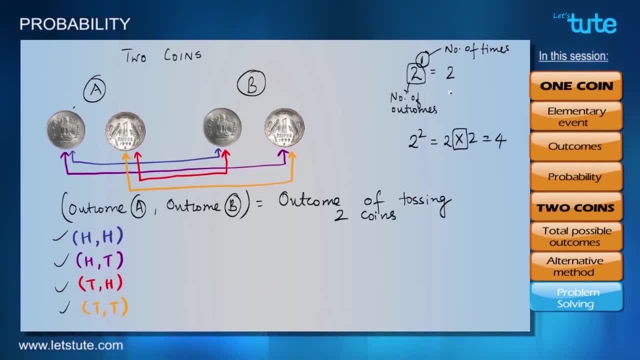 why multiplication and why not two plus two? the reason is we know that outcomes of a coin are mutually exclusive in nature, that is, when one appears, the other will not appear. but when we are tossing two coins, this event of tossing two coins are actually independent of each other, which means whatever outcome. 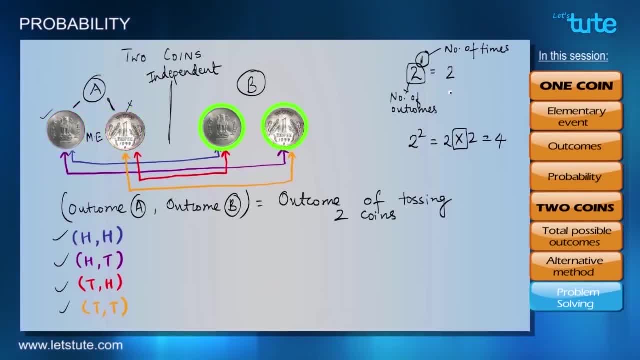 will appear on coin a. it will not interfere with the appearance of outcome from coin B. so whenever it is independent event we have to multiply. Similarly, if there were three coins, let's say coin C, which will again have outcome heads and tails, then the total possible outcomes. 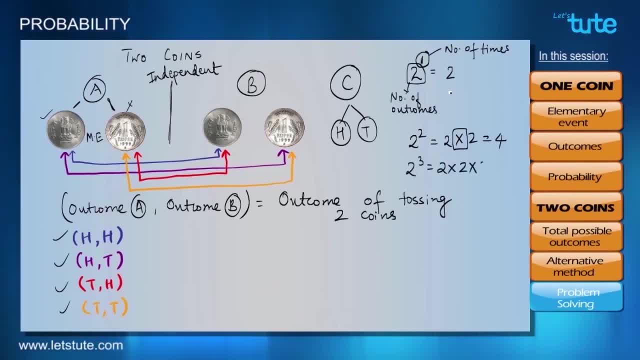 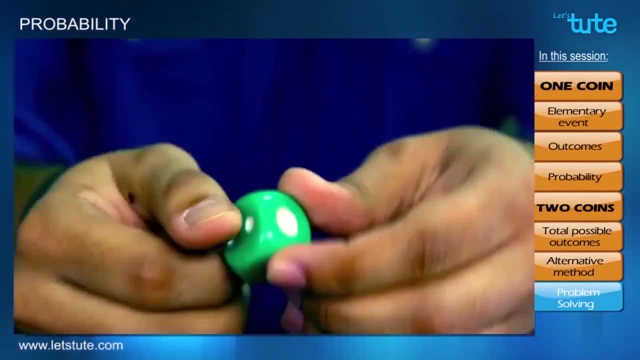 will be 2 raised to the power, 3 equal to 2 multiplied by 2. multiplied by 2, equal to 8, and not 2 plus 2 plus 2 equal to 6.. Similarly, in case of a die, we know that there are six. 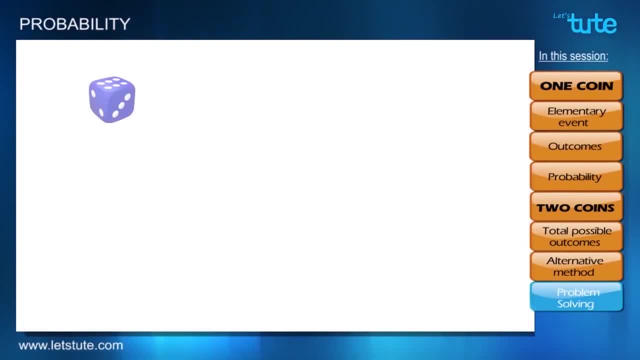 sides to one die. So these are the six possible outcomes. It is nothing but 6 raised to power 1.. Similarly, if we are throwing 2 die, then we will multiply the outcome from both and three die. again, it will be 6 multiplied by 6. multiplied by 6, equal to 6 cube. So we have 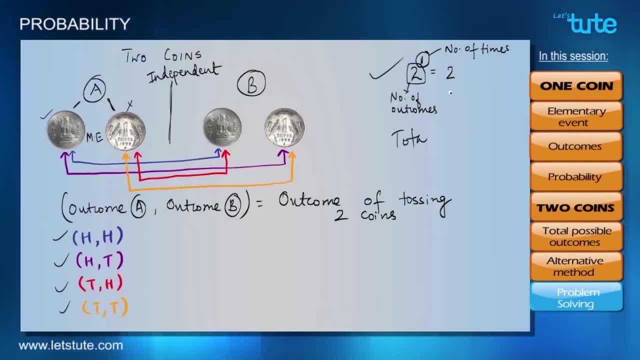 to remember this particular method in order to calculate the total possible outcomes faster. Now suppose we were to find out the probability of die getting exactly one head upon tossing two coins. so how will we go about it? so we know that there are total of four possible outcomes and we can see in 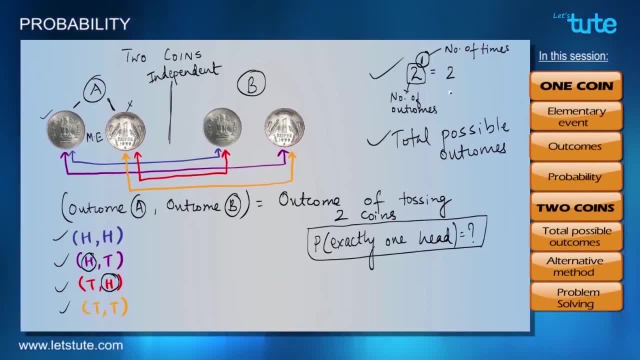 outcome number two and outcome number three. we have exactly one head, so the probability is two out of four, that is, one by two. we can certainly not take the outcome number one because there are two heads in the first outcome. similarly, if we were to find the probability of exactly one tail instead, then we can see. 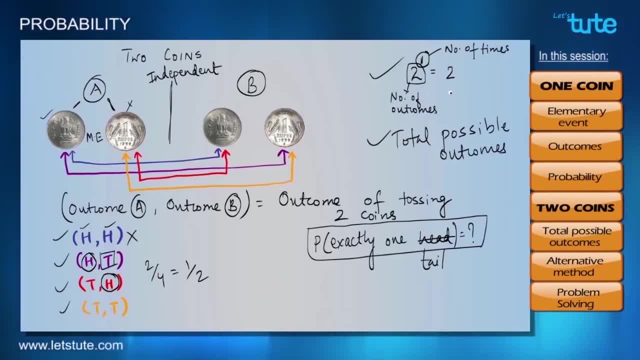 that we have one tail in outcome number two and in outcome number three, so the probability is again going to be one by two and we certainly cannot take fourth outcome because again we have two tails in it. in the same way we can work out probabilities associated with three coins, and we can play around all the.